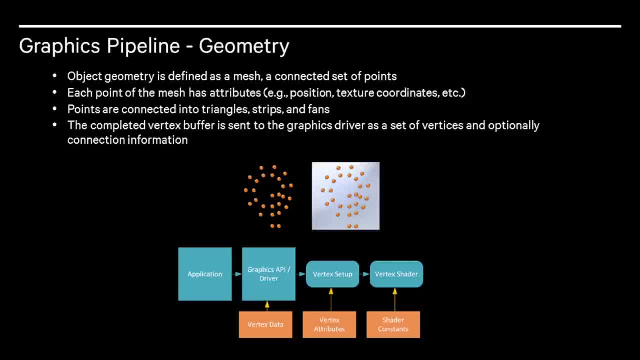 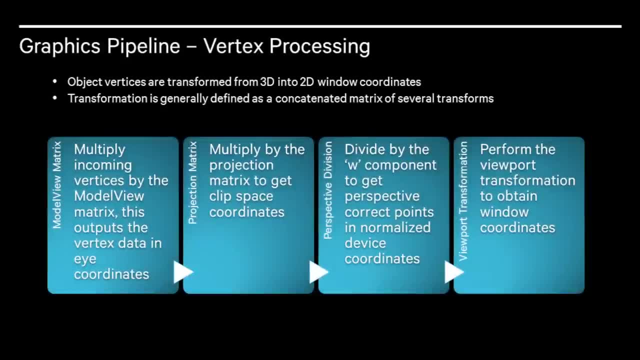 to the graphics driver to be rendered. The graphics driver is a low level library that commands the graphics hardware and implements a high level graphics API. The vertex shader is responsible for transforming the vertices from object coordinate space to window coordinate space. You can think of this as projecting points onto a 2D plane. 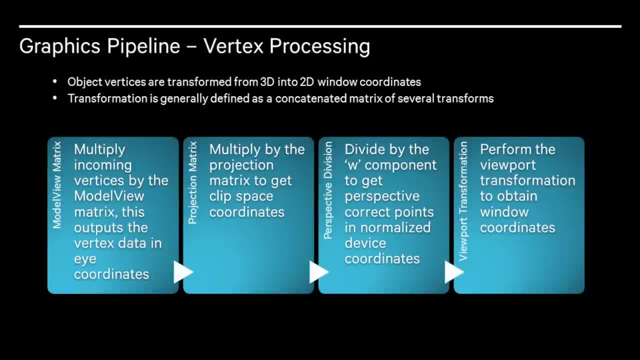 Traditionally this is done efficiently by performing a single matrix transformation of the vertex position. The matrix is calculated by concatenating several matrices together. These matrices convert each vertex from object coordinate space to eye coordinate space or camera coordinate space to normalize device coordinate space and then from there from. 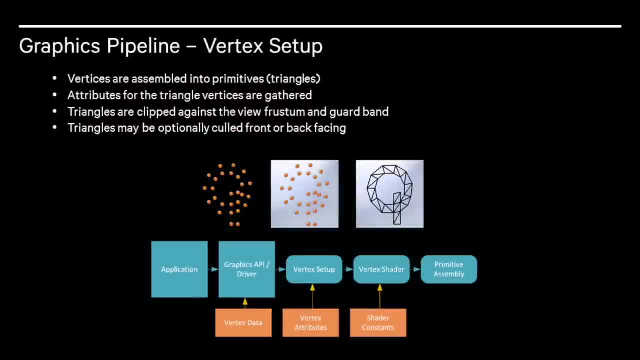 finally to window coordinate space. The driver assembles the transformed vertices into triangles. This is either done with the ordering of the vertices or with a separate buffer describing the connection of the mesh. Attributes for the vertices are collected as well. The triangles are then clipped against the frustum and the guard band Triangles. 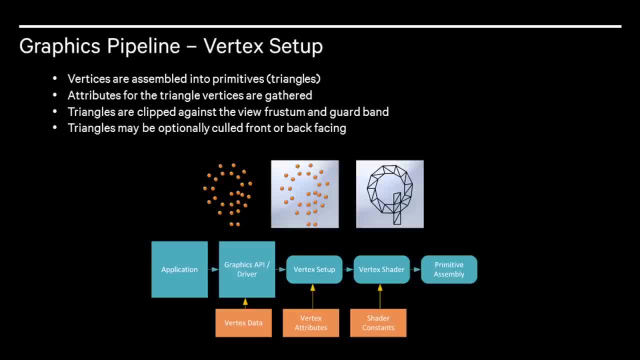 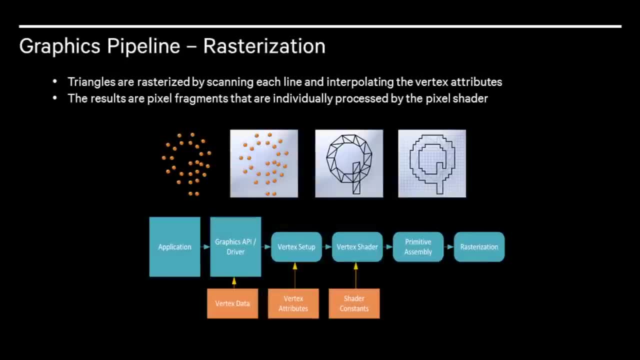 can be optionally culled and removed if they are front or back facing. Now the graphics hardware rasterizes the triangles. A scanline algorithm, which works by processing the triangle row by row, is generally used. Each pixel, now called a fragment which is covered by the triangle, is then sent to be further processed. Attributes for the fragments. 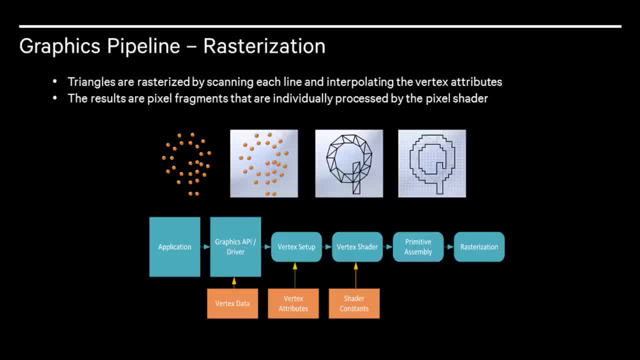 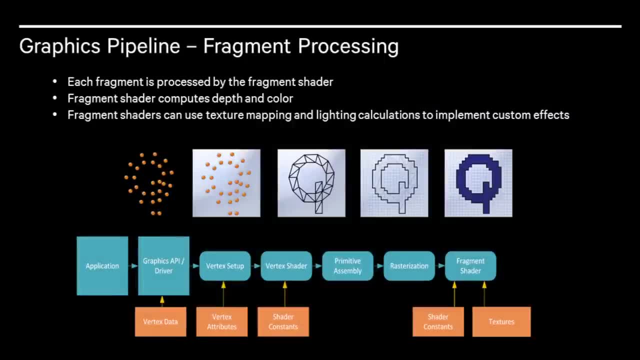 are also calculated by linearly interpolating the values from each of the three vertices. The fragment shaders, where the color of the pixel and the depth of the pixel are calculated and written to buffers. Fragment shaders are complex shaders that combine textures, lighting calculations, material properties and sometimes post-processing effects. 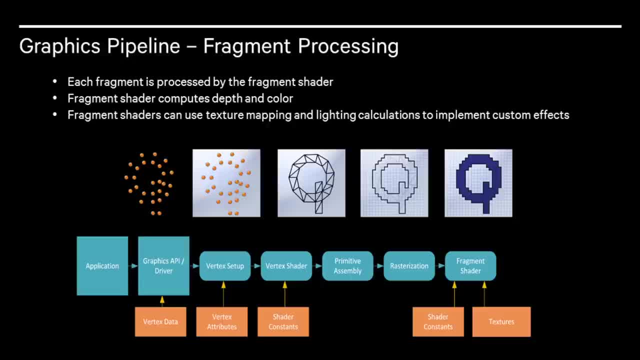 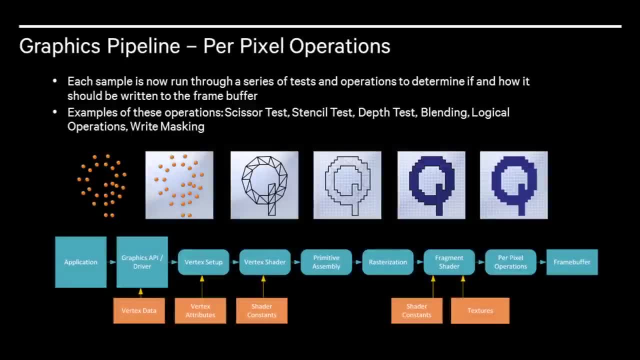 Once this step is complete, the fragment is passed on to the final step. Per-pixel operations are where testing and blending occur for the final pixel. Depending on the state set in the graphics API, the pixel is written to the framebuffer. An example: 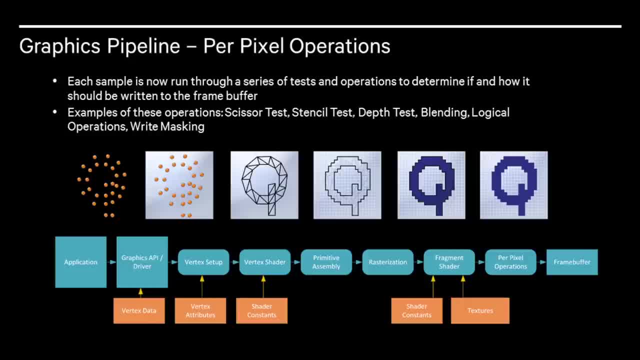 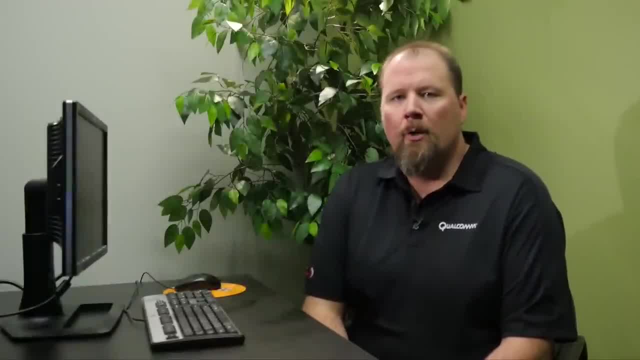 of this would be alpha blending. The pixel is blended with any existing pixels based on the alpha value. Let's talk about the evolution of the pipelines for a little bit. In OpenGL ES1, the pipeline was fixed. Essentially, you could switch things on or 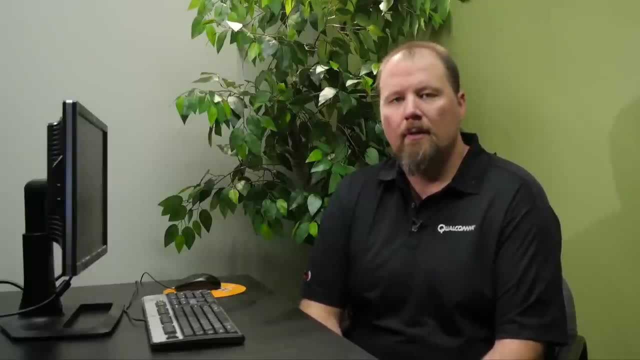 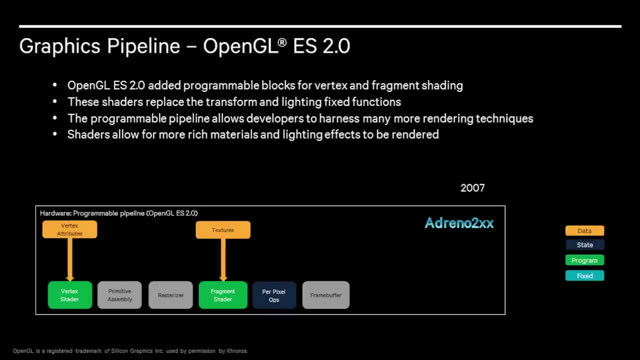 off, but it was impossible to custom program the pipeline In OpenGL ES2, it was a significant milestone for mobile graphics. Custom vertex and fragment shaders allowed a programmer to customize the pipeline. Some of the important features added in OpenGL 2 are programmable. 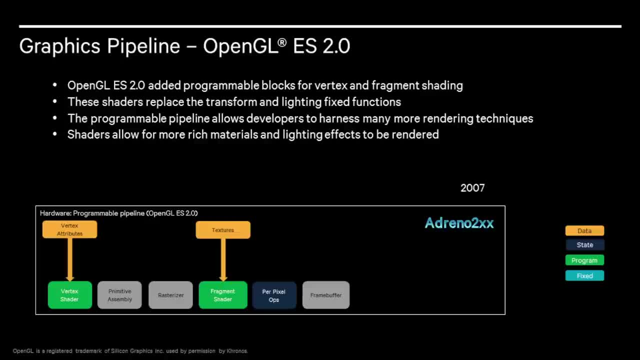 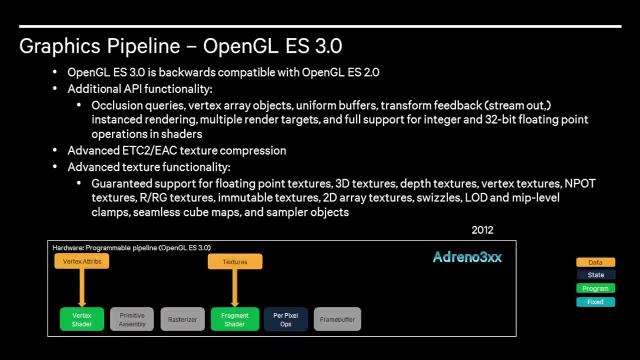 blocks for vertex and fragment shading. These shaders replaced the transform and lighting fixed functions that were normally switched on or off. The programmable pipeline allows developers to use many more rendering techniques and the shaders allow for much more rich materials and lighting effects. With OpenGL ES3, the next generation of graphics hardware allowed even more advanced features. 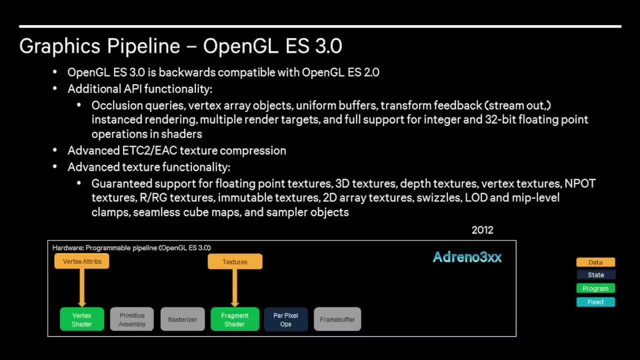 to be implemented in mobile games. GL ES3 is backwards compatible with GLE S2 and additional API functionality you can embed to OpenGL ES3 with occlusion queries, vertex array objects, uniform buffers, transform feedback instance rendering and multiple render targets with들을 and hetero BBC denkees, which of course are overrated with miscellaneous. 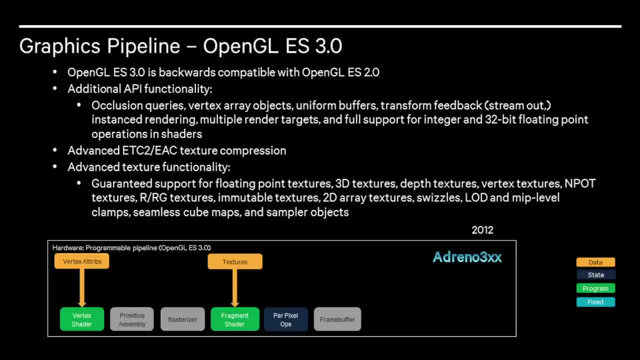 rendercciones que los findetan en estas y fases, and full support for integer and 32-bit floating-point operations and shaders. The API also introduced new texture compression formats called ETC2 and EAC. Also advanced texturing functionality, including guaranteed support for. 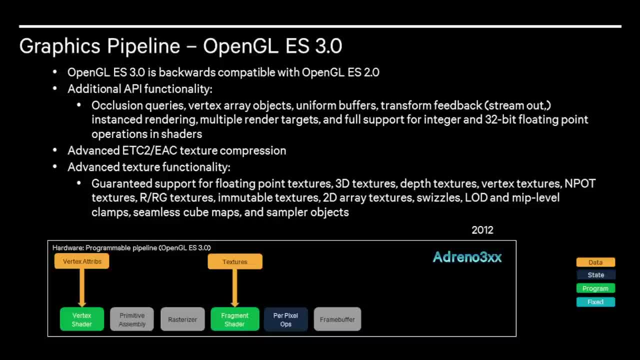 floating-point textures, 3D textures, depth textures, vertex textures, non-power of two textures, red and red-green, only channel textures, immutable textures, 2D array textures, swizzles, LOD and MIP level clamps, seamless cube maps and 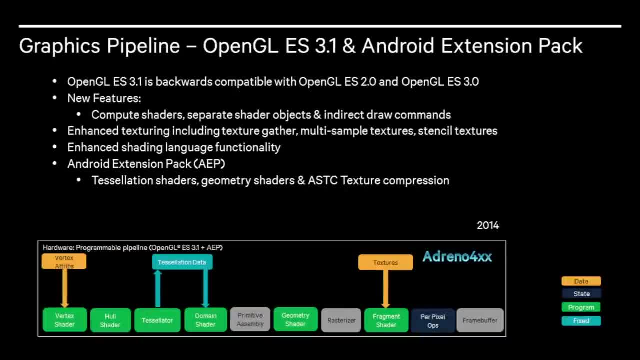 sampler objects. OpenGL ES 3.1 and the Android Extension Pack provide additional functionality to the developer. OpenGL ES 3.1 is backwards compatible with 3.0 and 2.0.. New features include compute shaders, separate shader objects, indirect draw commands, enhanced texturing, including texture gather. multi-sample textures, stencil textures and same-sex texture gathering. The APIs also introduced a new feature called OpenGL ES 3.1.. The API also introduced a new feature called openGL ES 3.1.. The API also introduced a new feature called. 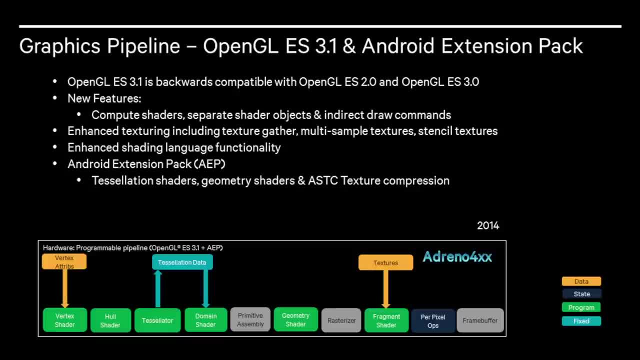 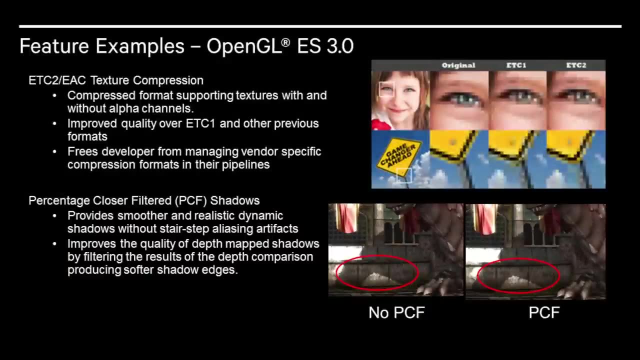 enhanced shading language functionality. The Android extension pack is a set of new extensions over GLES 3.1. New features in that include tessellation shaders, geometry shaders and ASTC texture compression. Next let's cover some of the practical examples for version 3 of the OpenGL ES API. First, it 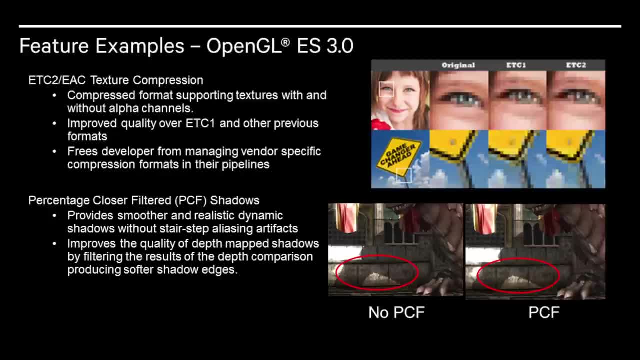 added ETC2 and EAC texture compression. This is a compressed format supporting textures with and without alpha channels. It has improved quality over ETC1 and other formats. It is a standard texture compression method that makes development easier on Android. You are no longer required to use vendor-specific 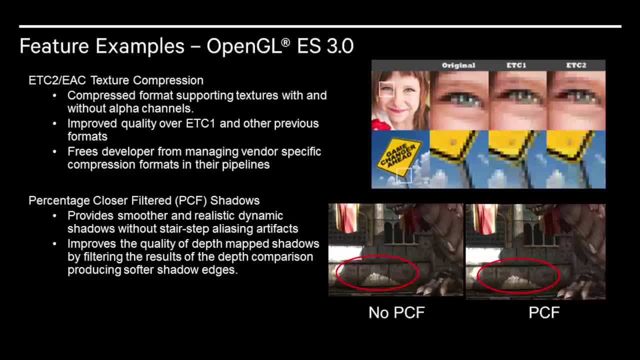 compression formats in your pipelines. It also added percentage closer filtered shadows. They provide smoother and realistic dynamic shadows while filtering out much of the aliasing artifacts. Improves the quality of depth map shadows by filtering the results of the depth comparisons shown here. It changes the pigmentation of shadows by adding new. 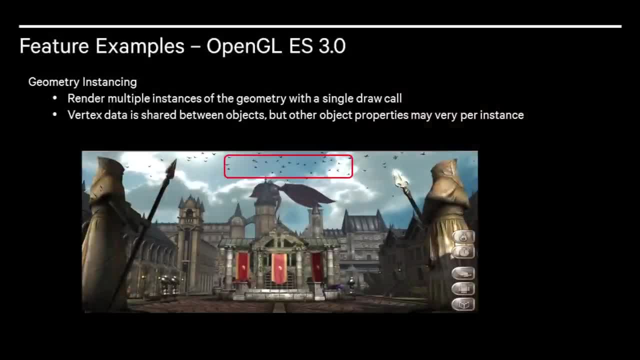 comparison, producing softer shadow edges. Another powerful feature is geometry instancing. With instancing, you can render multiple instances of the geometry with a single draw call. Vertex data is shared between objects, but other object properties may vary. per instance, Instancing is especially important on mobile GPUs. 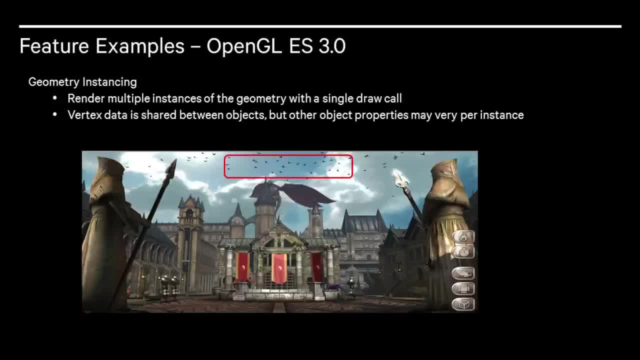 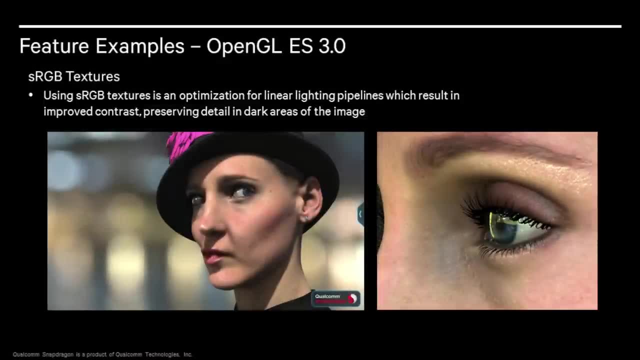 where there is typically a high CPU overhead per draw. call GLE S3 also added support for sRGB textures. Using sRGB textures is an optimization for linear lighting pipelines, which results in improved contrast while preserving detail in dark areas of the image. 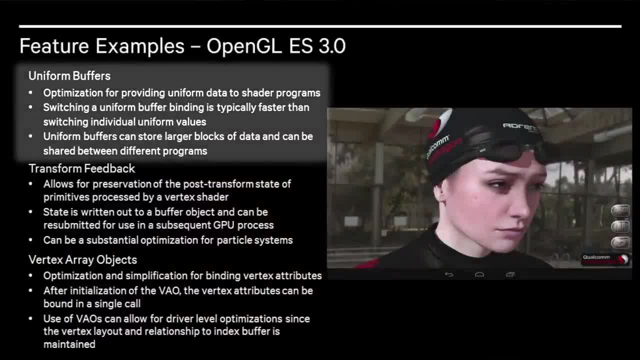 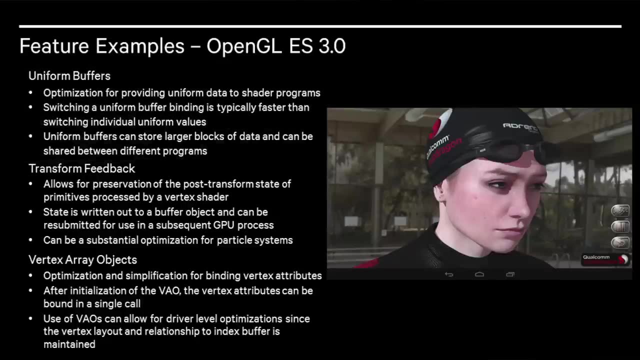 Uniform buffers. This is an optimization for providing uniform data to shader programs. Switching a uniform buffer binding is typically faster than switching an individual uniform value. Uniform buffers can store larger blocks of data that can be shared between different programs, like a matrix, transform, et cetera. 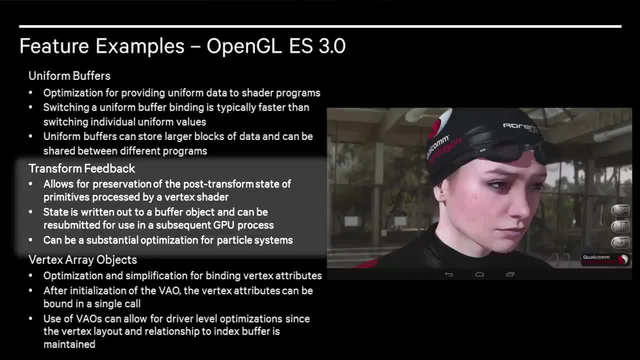 Transform feedback. This allows for the preservation of the post transform state of primitives processed by a vertex shader. State is written out to a buffer object and then can be resubmitted for use in subsequent GPU processes. This can be used as a substantial optimization.